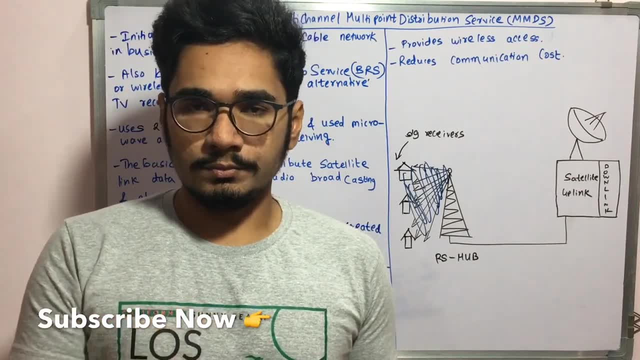 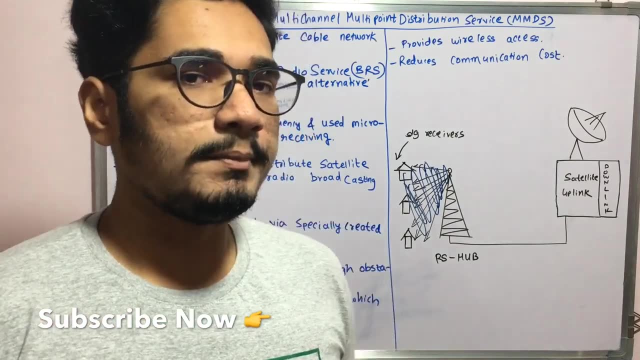 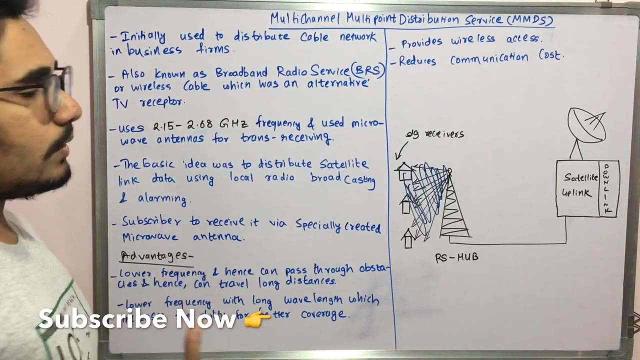 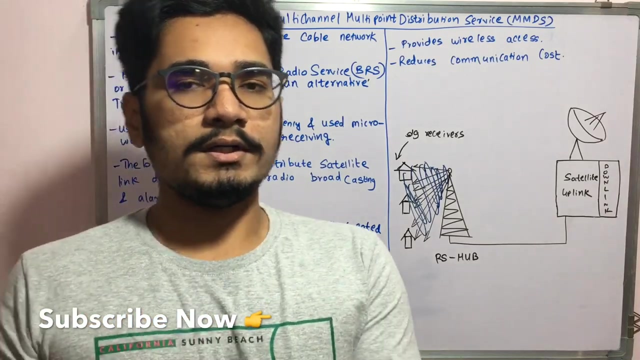 So it is wireless. Now, in the recent days it's also been used in the television systems where TV receptors are being configured in order to accommodate this MMDS service. So it's also known as broadband radio service, BRS or wireless cable, which is an alternative to the television receptor. So, in place where the older televisions had the older chips and cathode, ray tubes, CRT and all, So in the modern television it's being 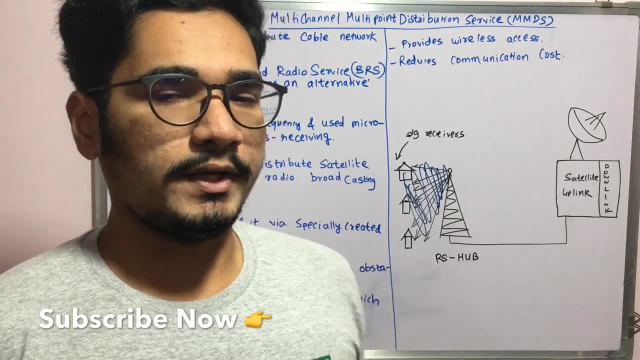 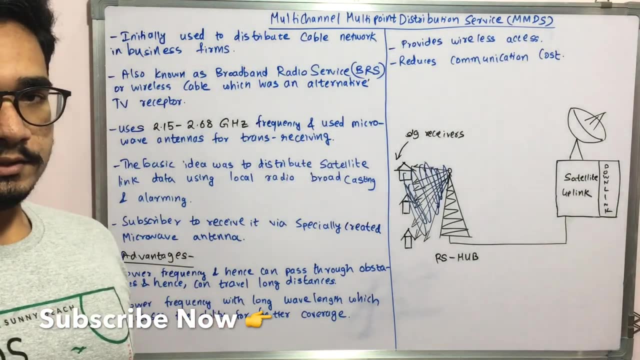 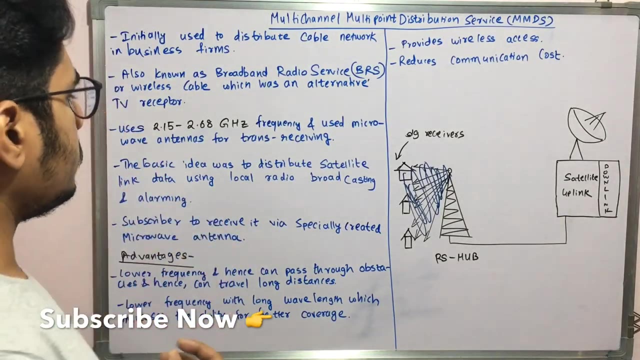 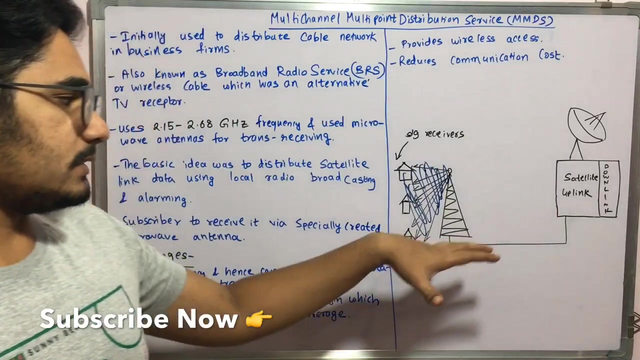 configured with these systems which is capable of MMDS receiving, and so it's called as the broadband radio service, BRS. So now this MMDS operates or uses with the frequency range of 2.15 to 2.68 GHz and is used in microwave antennas for a trans receiving. So the antennas or the broadcasting station which it has basically has microwaves got and it transmits the microwaves which reaches 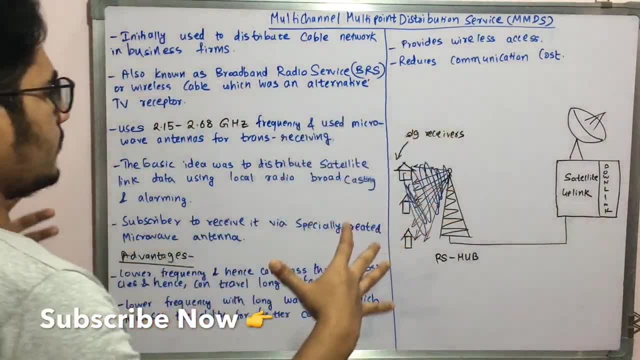 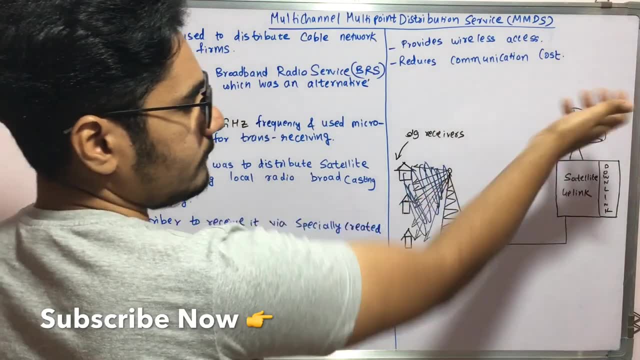 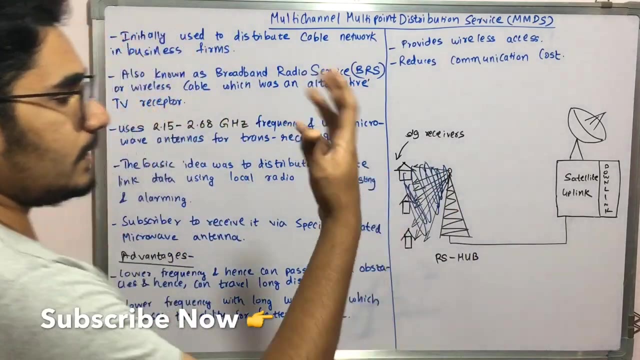 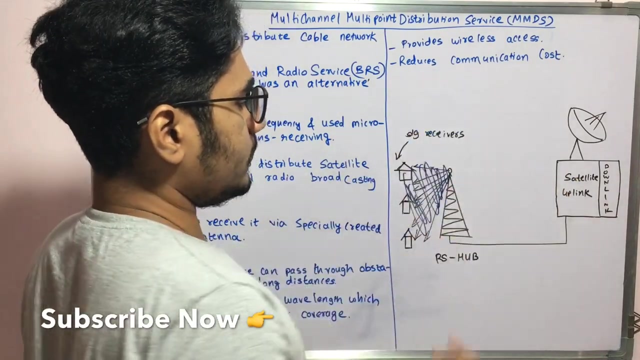 to each of the signal receivers. So the basic idea here is: so the setup is of MMDS is something like this. So the basic idea here was to distribute the satellite data. So you have the satellite. So satellite will have two kinds of links, that is, satellite uplink and satellite downlink. So mainly the satellite uplink data needs to be transmitted to each of the signal receivers, and so it is done by means of an RS hub, which is a broadcasting station, and then with the help of RS hub. 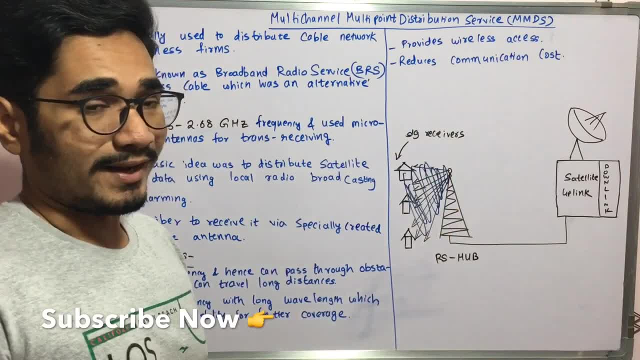 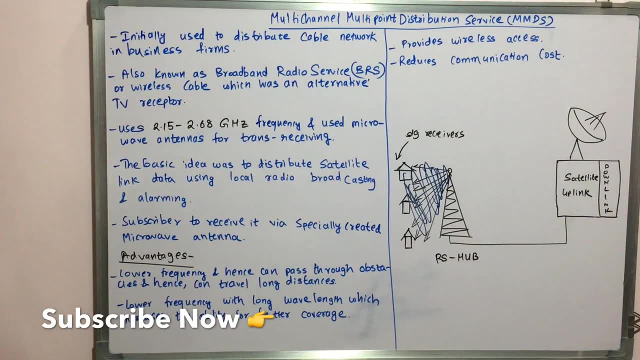 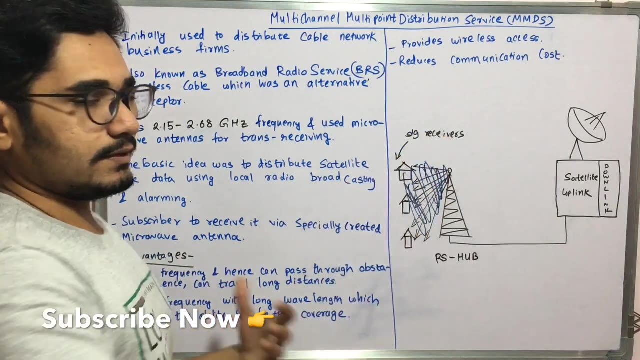 hub or broadcasting station. it used to transmit each of this microwaves to each of this individual signal receivers. so the subscriber is used to receive it. specially created microwave antenna. so this microwave antenna- specially this- is being user created or depending upon the area, location or geographical location. 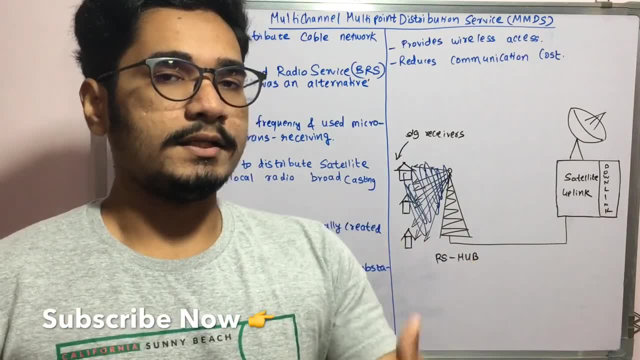 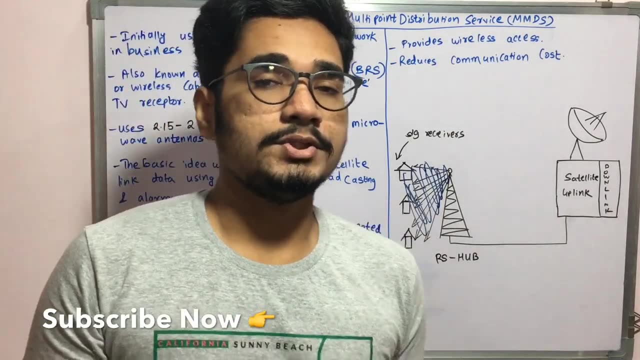 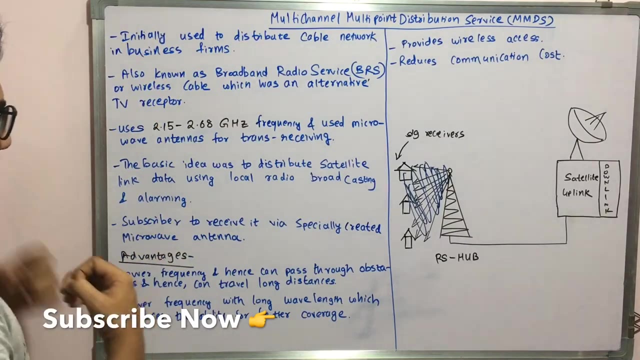 this is being configured. it's not a standard particular antenna that you can just install and make it work in all the places, but then you need to know the geographical conditions or what conditions are there in that particular area. so it has got few of the advantages. so, since it's of lower frequency and hence can pass through obstacles, and thereby it can travel longer distances. so since its microwaves, its collision with the hard objects is very less, and so with that it can travel to to even much more longer distances. then the lower frequency with long wavelength, which increases the ability for better coverage.